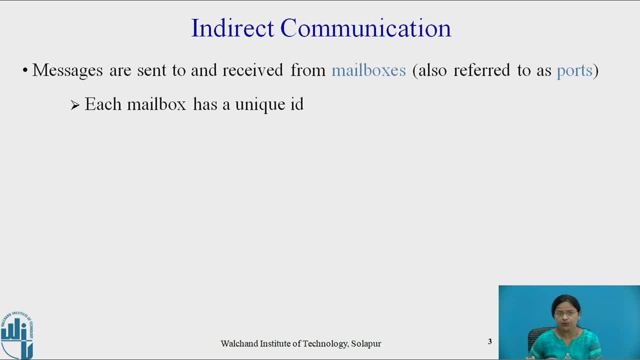 as an object where messages can be queued by the processes and the messages can be removed by the processes. so the mailbox has an unique identification number. the processes can communicate with each other only if they share a mailbox. the two process can communicate if they have a common mailbox shared with them in. 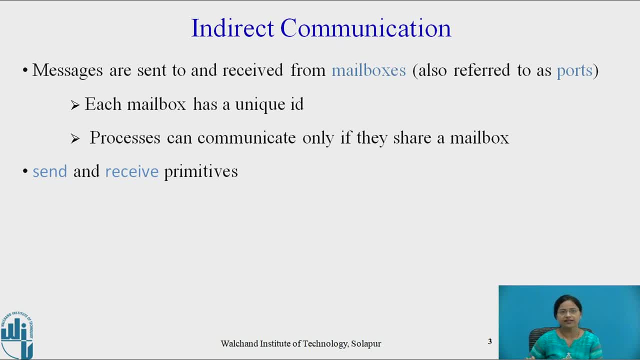 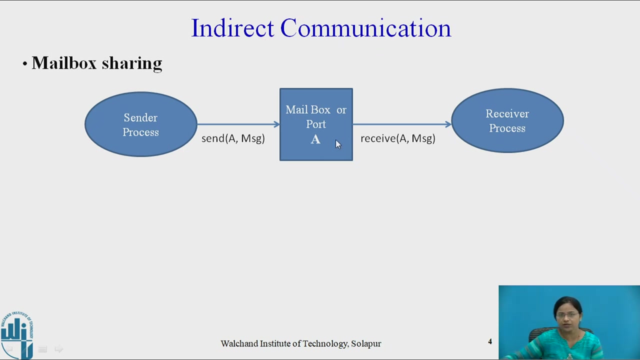 indirect communication: send and primitives are sent and receive. primitives are used. the same primitive is: send a comma message means send a message to mailbox a and receive a comma message means receive a message from mailbox a, so mailbox sharing text place like sender process. here sender process sends a message to particular mailbox a or port a and receiver process receive a. 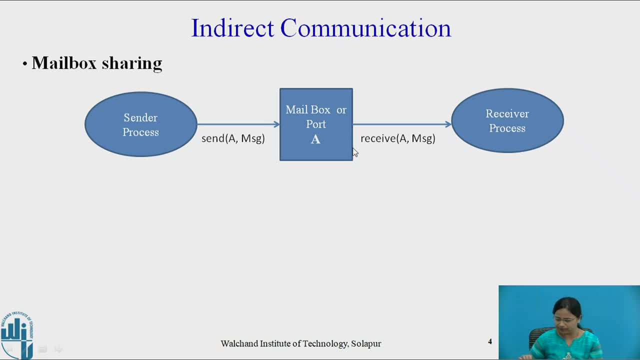 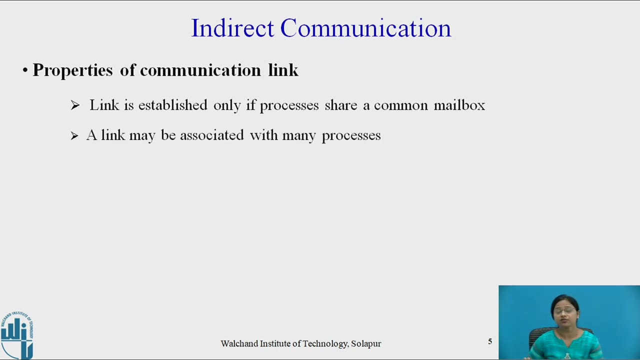 message from that mailbox or port a. this is indirect communication. the properties of communication link in indirect communication are: link is established only if processes share a common mailbox. a link may be associated with many processes between each pair of communicating process. a number of processes may be associated with many processes between each pair of. 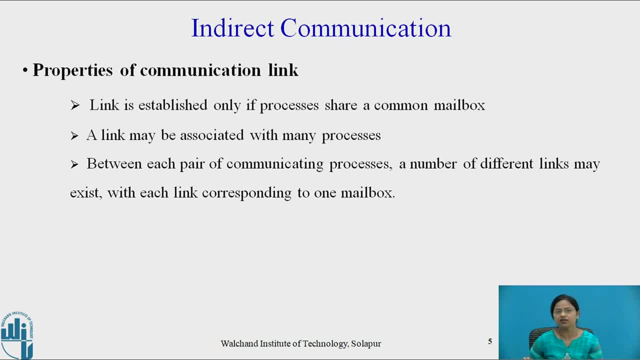 different links may exist, with each link corresponding to one mailbox. So though, there are multiple pair of communicating processes, but each two process must share common mailbox. Link may be either unidirectional or bidirectional. Unidirectional means sometimes we get mail from no reply. 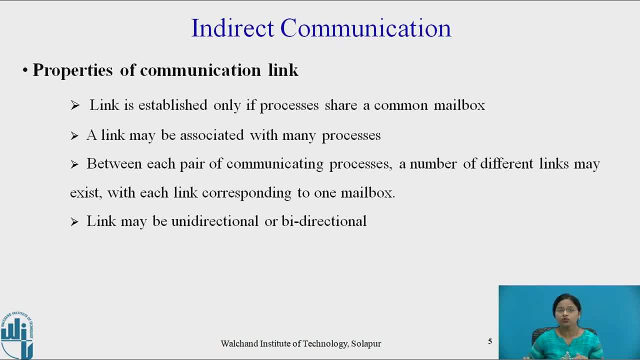 So there are some mailboxes which allow to send only message. They don't accept message from any other receiver. that is unidirectional. Bidirectional means we can receive a message from particular mailbox or we can send a message to that mailbox. So unidirectional means we get a message as a no reply. 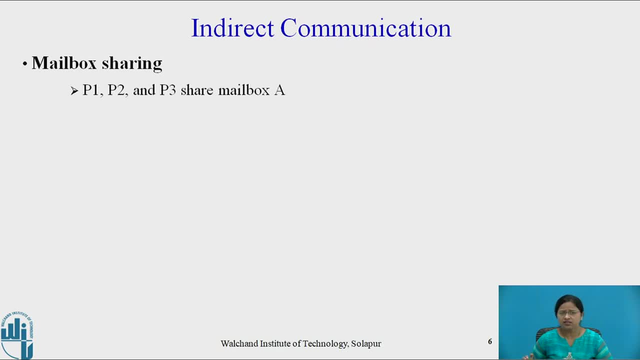 So the mailbox sharing here. suppose we have an example of three processes, P1, P2 and P3, which share a common mailbox A. P1 sends a message to mailbox A and P2 and P3 executes receive from A. Then who will get the message? 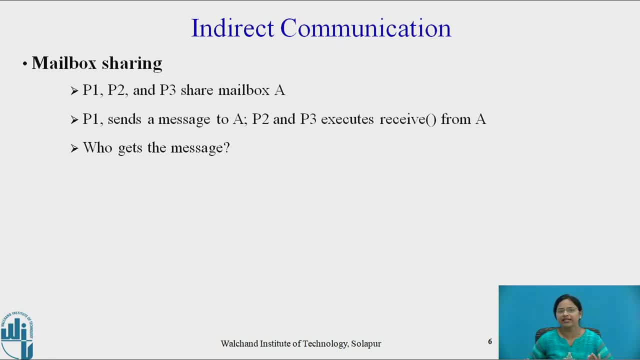 We know that both processes, P2 and P3- both will get the message, but this depends on the method used by the operating system. So operating system may allow a link to be associated with at most two processes So that the message can be sent to two process. 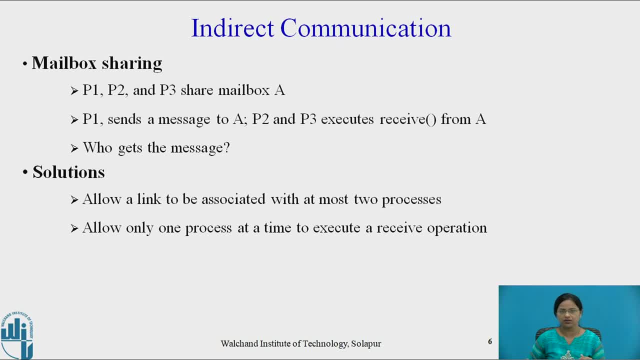 Allow only one process at a time to execute a receive operation means, though, there are multiple processes in the system which wish to receive a message, but OS will allow only one process at a time to receive a operation or allow the system to select arbitrarily the receiver, or system may select a receiver process randomly, and sender is notified who. 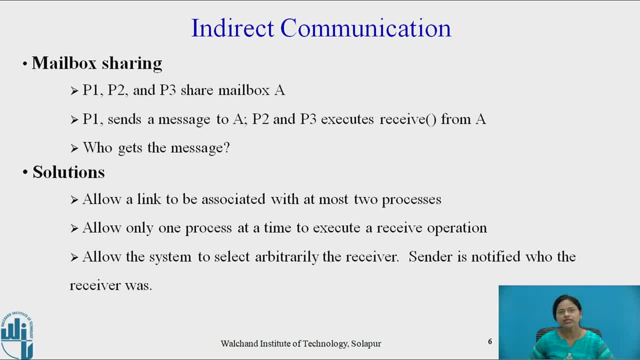 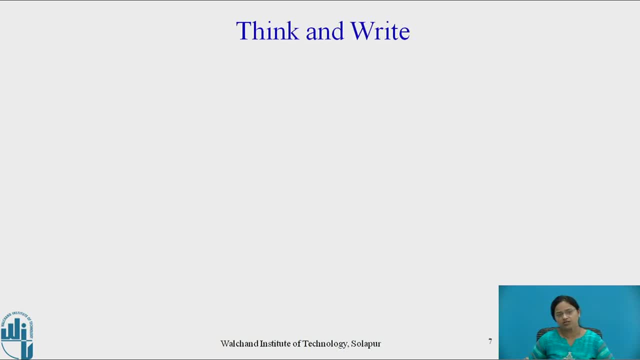 the receiver was and it sends the notification to the receiver, to the sender to whom the message was sent, P3.. Now just pause the video and think that in our daily life, where we use this inter-process communication, pause the video and just think on it. ok, let us see the answer, the most important. 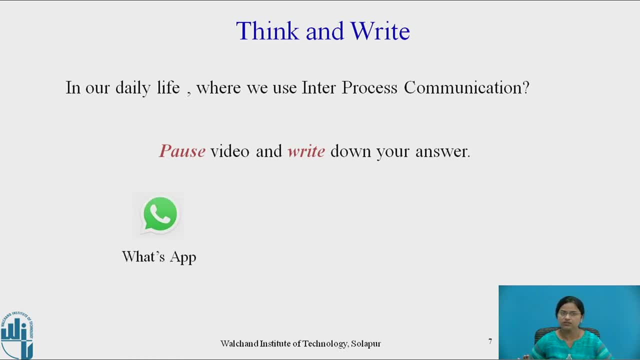 thing which we use is whatsapp. using whatsapp, we share messages with each other. ok, we share a message with group or we can share a message. we can share a message personally also. the second example is email mailbox. we are, we have a mailbox and we get the message from. 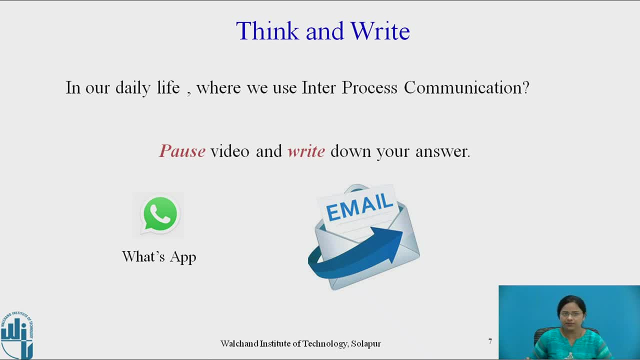 different mailboxes. ok, there are many examples of this inter-process communication which we use in our daily life, but whatsapp and email are the most commonly used inter-process communication technique or application P4.. Now let us see the second example, P5.. Now, in the inter-process communication, the processes communicate with each other using 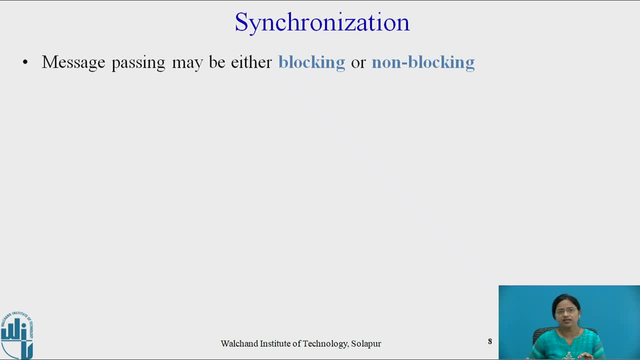 send and receive primitives. ok, so that send and receive primitives can be implemented in different ways. so message passing using send and receive may be either blocking or non-blocking. so blocking is considered as a synchronous and blocking has two types. blocking send means the sender is blocked until receiver receive the message. 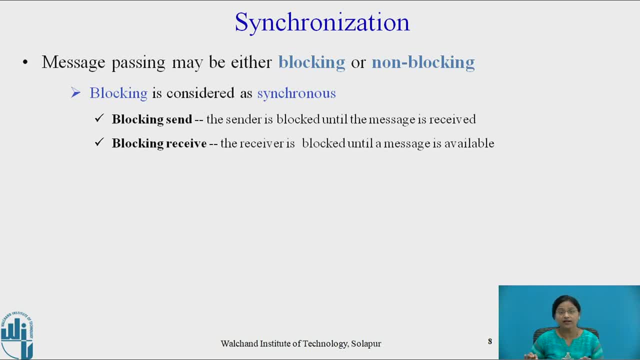 And blocking. receive means the receiver is blocked until a message is available. The next type is non-blocking. non-blocking is considered as a asynchronous. non-blocking send means sender sends message, but it doesn't wait. it continue with its own operation. it doesn't wait whether receiver receive an operation or not. non-blocking receive means here the 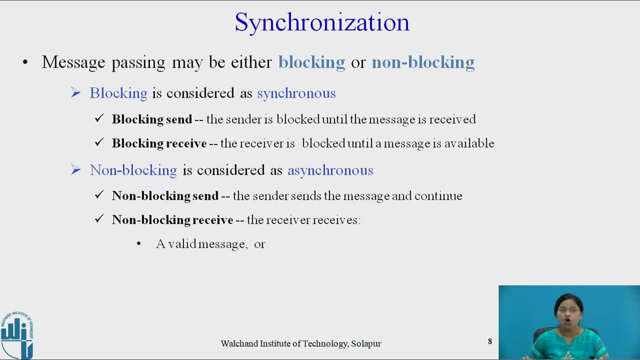 receiver receives a message, but that message may be a valid message or it may be a null message. Now, blocking send, blocking receive, non-blocking send and non-blocking receive. these four, these four type exist. blocking is called as synchronous because here sender wait till receiver receives a message, while this is called as asynchronous. why? because sender sends a message and it. 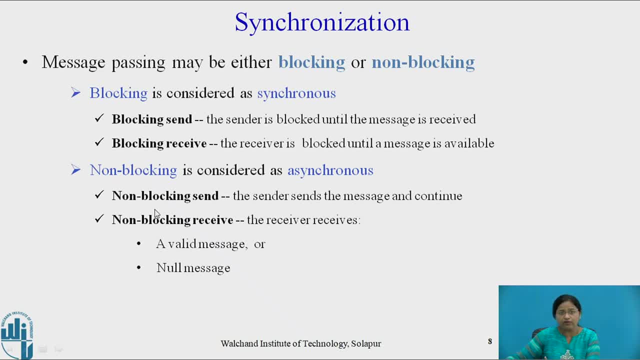 doesn't wait. so this: this may have different combinations, so different combinations may be possible using these four. So if anyone selects Both sender and receiver as a blocking, then the system may be randosius means here, suppose a producer and consumer. if we select producer process, also blocking and consumer process. 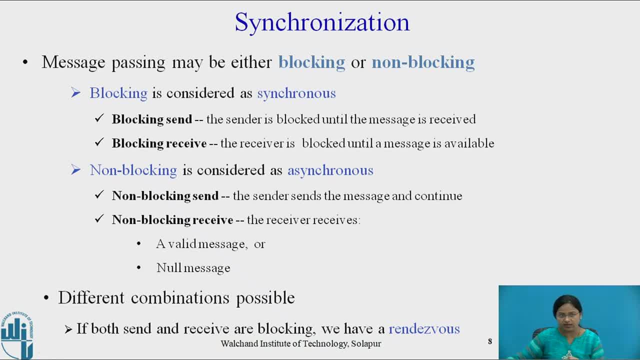 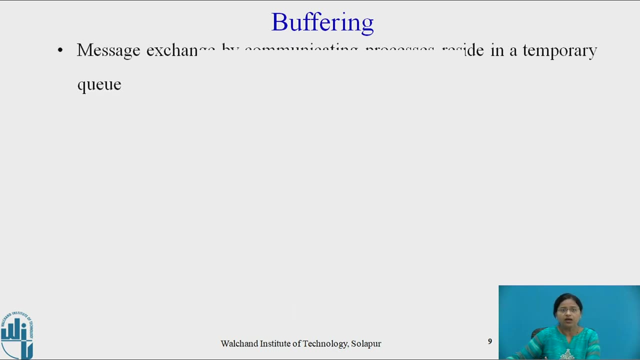 also blocking. producer will wait till consumer consumes an atom and consumer will wait till producer produces an atom. so in this case both may go in waiting. state and system may result in randosius situation. Next is buffering. Now, In buffering the communication may be direct or indirect. the message exchange by communicating. 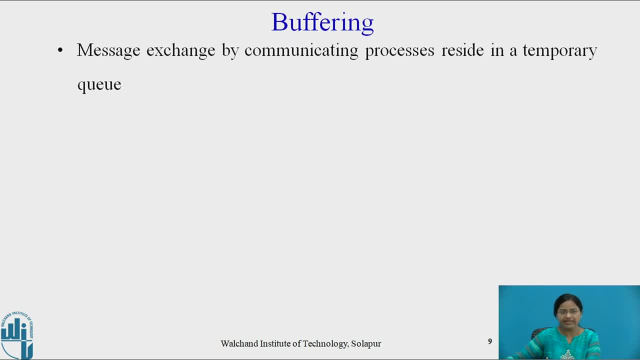 process reside in temporary queue. so queue can be implemented in three ways. first is zero capacity. in zero capacity, queue has maximum length. zero link cannot have any message waiting in it. sender blocks until the recipient receives the message. so here blocking send is used. ok, so the application of this zero capacity is used in handshaking. 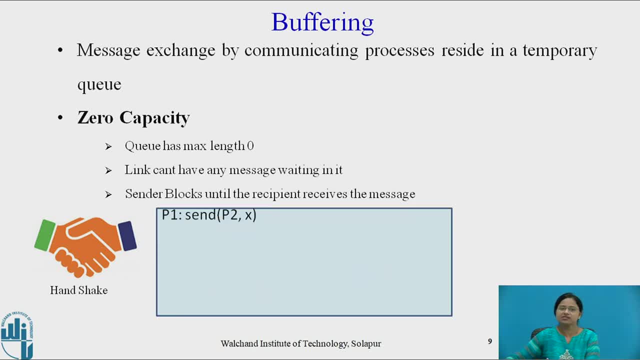 Here: suppose process p1 send a message to process p2, p2 receive a message from process p1. here, when process p1 send a message, it will block till p2 receives a message. once p2 receive a message, p2 send a message to process p1 and when p2 send a message, it wait till p1. 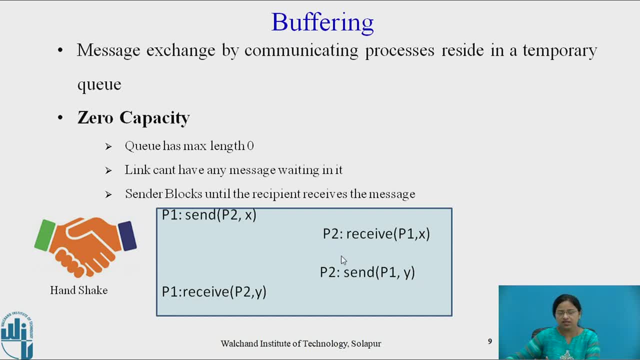 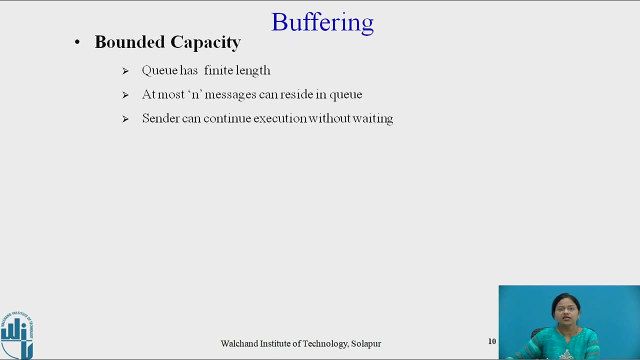 receive a message. so in this case both sender and receiver are blocking. this type of operation is used in handshaking, where one to one communication takes place. Next type is bounded capacity. in bounded capacity, queue has finite length. at most, n number of messages can reside in queue. sender can continue execution without waiting. so example of this: 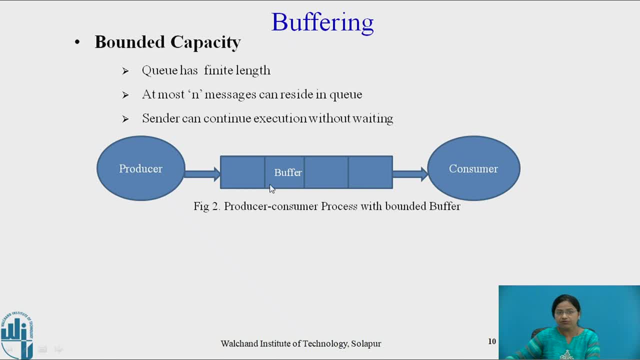 is producer- consumer process with bounded buffer. now buffer has some fixed size. producer produces an item If Space Space is available in buffer and consumer consumes an item if item is available in buffer. producer will wait only when buffer is full and consumer will wait only when buffer is. 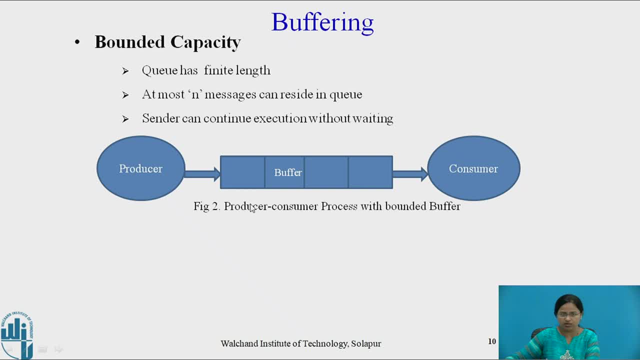 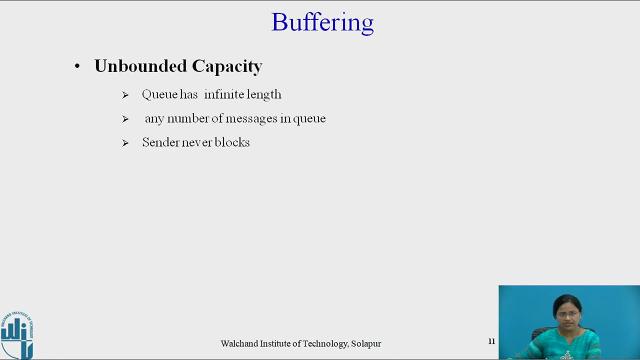 empty. so this is one example of bounded capacity producer consumer problem. second example is sender process: send a message to mailbox a and receiver receive a message from mailbox a. so these two are examples of bounded capacity. third type is unbounded capacity. in unbounded capacity, queue has infinite length. any number of messages may reside in queue and sender. 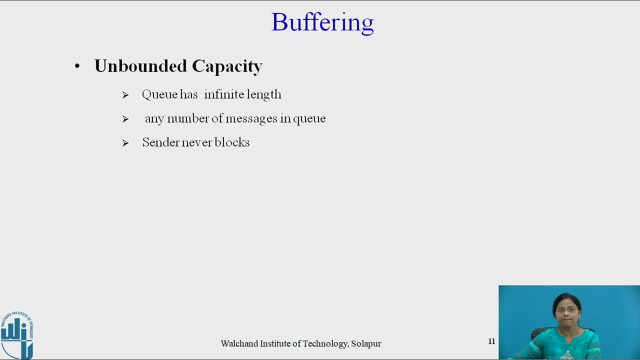 never. block sender will continually send message to the queue. example of this: there may be only one producer and n number of consumers may present there. there may be n number of producers and only one consumer will be there, and n number of producers may be there and n number of consumers may exist. so these are three types of buffering for inter process. 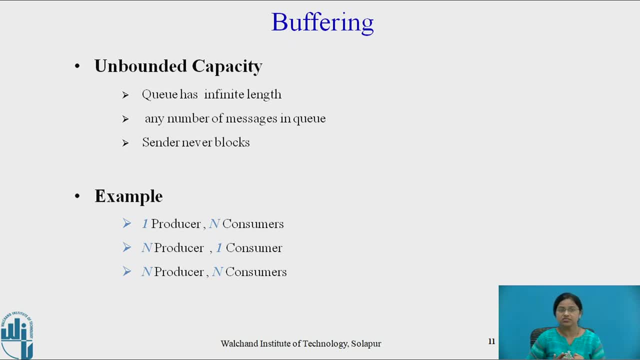 communication technique of message passing, where zero capacity is also called as no buffering, while bounded capacity and unbounded capacity is called as automatic buffering. you so in this video, we studied how message passing is used for indirect communication using mailbox and how buffering technique takes place. how buffering technique is used. 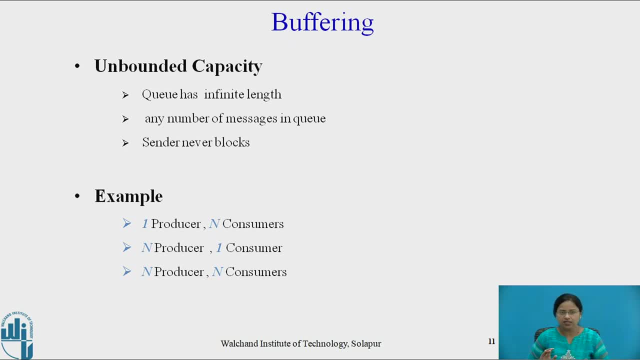 for implementing this message passing system for indirect communication. Thank you. These are the references. thank you.